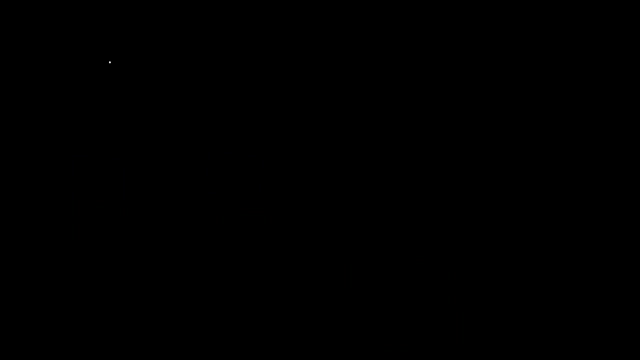 10 over 3.. Now let's try another example: 3 over 5, divided by 1 over 4.. Feel free to pause the video and try that example. So let's keep the first fraction the same and then let's change. 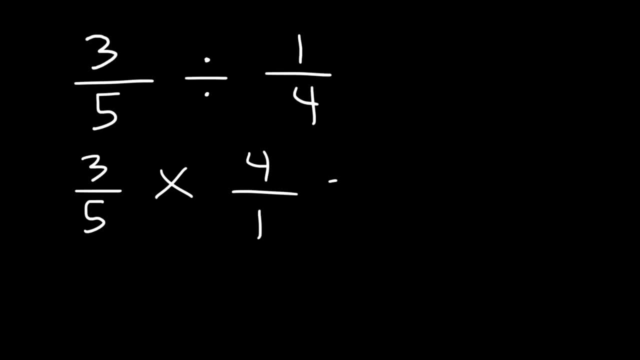 division to multiplication, and then we're going to flip the second fraction and then multiply across. So 3 times 4 is 12.. 5 times 1 is 5.. Now we can't reduce this fraction, so this is going to be the final answer: It's 12 over 5.. 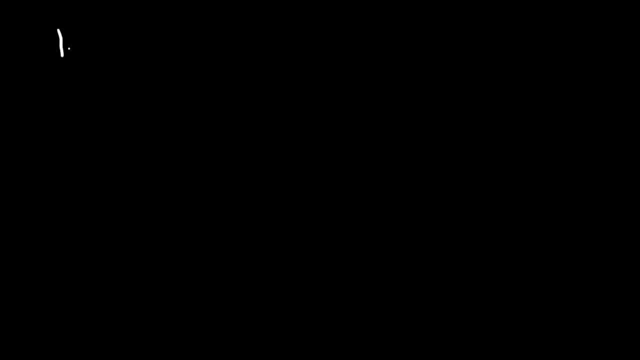 Now let's try an example with large numbers. So let's say, if we have 12 over 21 divided by 16 over 28.. So feel free to pause the video and work on that example. Go ahead and give it a shot. 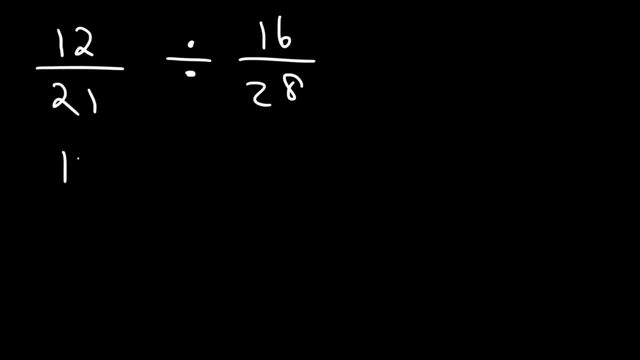 So let's keep the first fraction the same And, as always, let's change division to multiplication, and then we're going to flip the second fraction. Now, when multiplying two fractions, if you have large numbers, it's better to simplify before you multiply. We can rewrite 12. 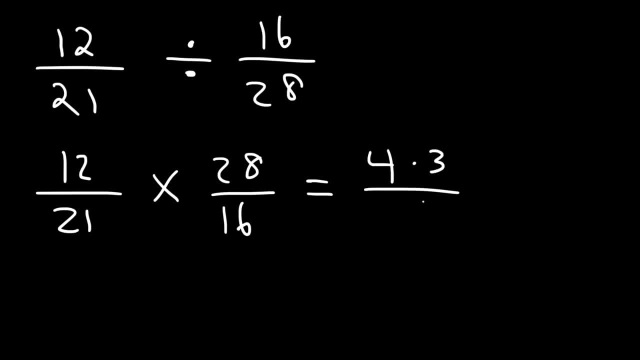 as 4 times 3 and 21. that's basically 7 times 3.. 28- we can rewrite that as 7 times 4.. And 16 is 4 times 4.. So we can cancel a 7,. we could cancel the 3,, we can cancel a 4,. 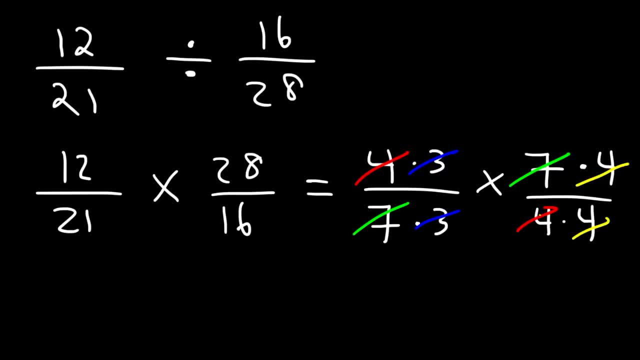 and we can cancel another 4.. When everything cancels, your answer is a 1.. If you think about it, 3 divided by 3 is 1.. 4 over 4 is 1.. So the whole thing is simply 1.. Now let's move on to our 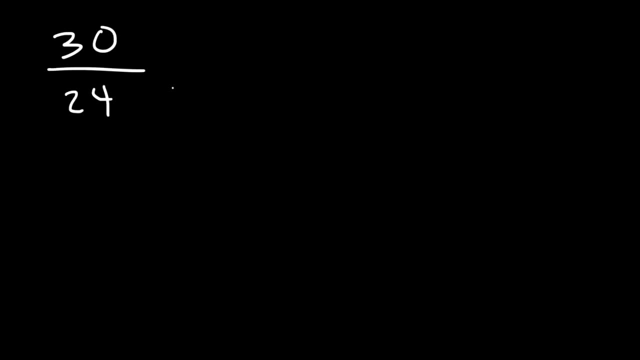 next example: and so it's going to be 30 over 24, divided by 45 over 72.. So go ahead and try that example. So let's begin by changing division to multiplication and by flipping the second fraction. So what can we break 30 into? So what two numbers multiplied to? 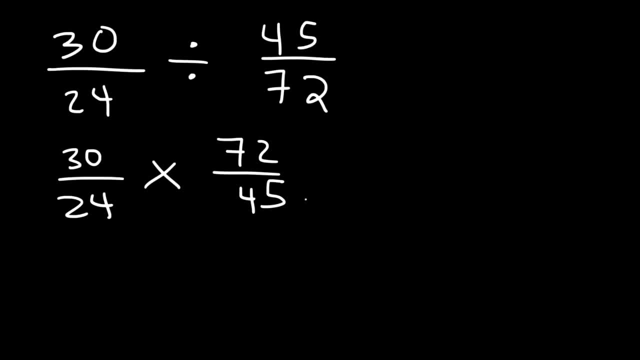 30? You could say 15 in 2.. You could say 10 in 3.. three, you can say six and five, but notice that 24 you can write that as six and four. so therefore we want to make 30 equal to six times five, because 24 we can make it six times four and we can cancel. 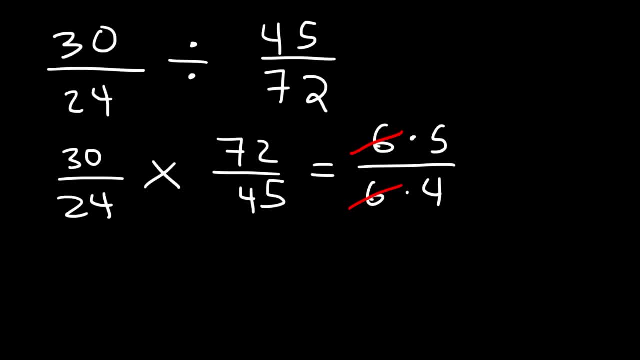 a six. so you always want to break down the numbers in such a way that you can cancel after you break it down. now, 72 and 45: they're both divisible by nine, so i'm going to write 72 as nine times eight and 45 as nine times five. so at this point i can cancel a nine and i can cancel a five. 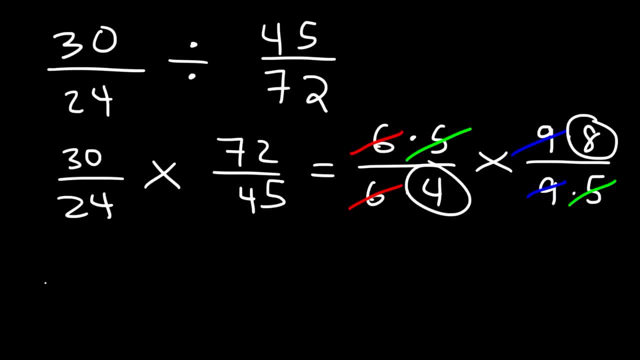 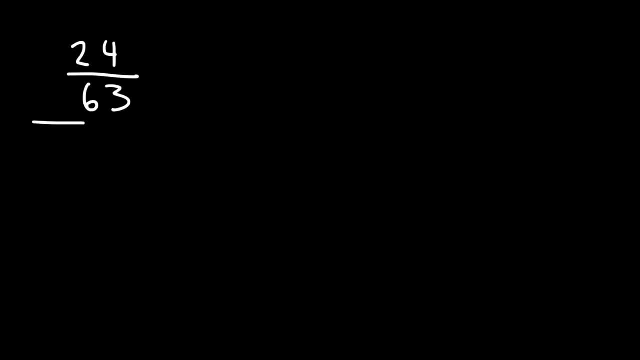 so i'm left with eight over four, and eight divided by four is two. so the final answer in this problem is two. sometimes you may need to divide two fractions in this form. so let's say, if we have a fraction over another fraction, so we have two fractions placed in one big fraction, how can we divide those two fractions? 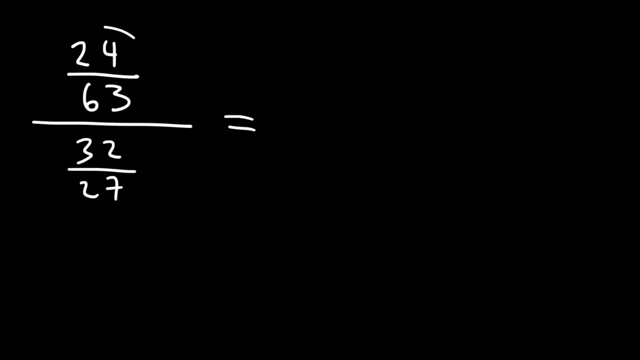 it's important to understand that this expression that we see here is equivalent to this expression. it's 24 over 63 and this big fraction means, divided by the other fraction, 32 over 27. so now it's in a form that we're more familiar with. so using keep, change, flip, it's going to be. 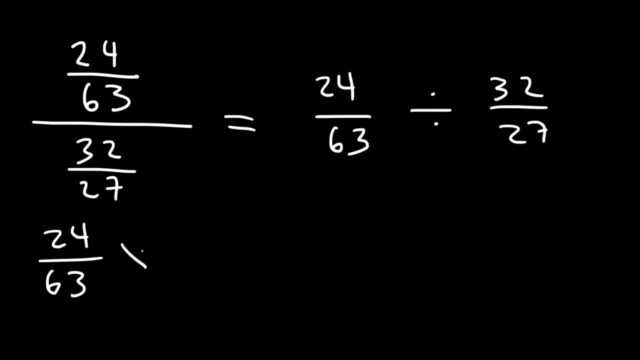 a 24 over 63 times the reciprocal of the second fraction, 27 over 32. so now we need to find a way, the best way, to basically break down these numbers so that we can cancel and get a final answer. so what? two numbers multiply to 24. we have 1 and 24, which is not going to help us. 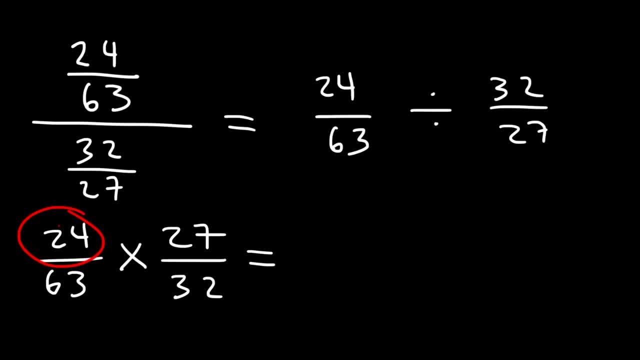 2 and 12, 3 and 8 and 6 and 4. now, looking at the 32, 32 is divisible by 8, not by 6. 8 times 4 is 32. so therefore i want to break down 24 into 8 and 3. 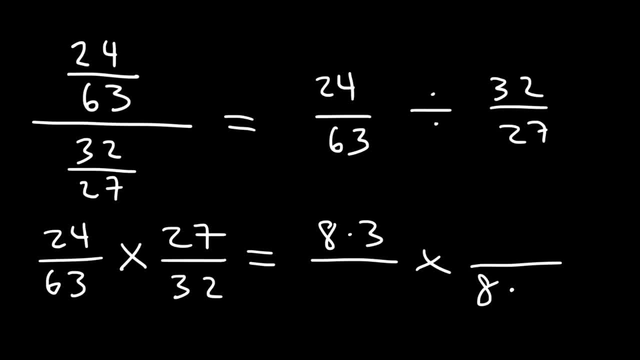 and 32 into 8 and 4, because i can cancel an 8. now, looking at 63 and 27, both numbers are divisible by 9. 63 is 9 times 7, 27 is 9 times 3, so i can cancel a 9. 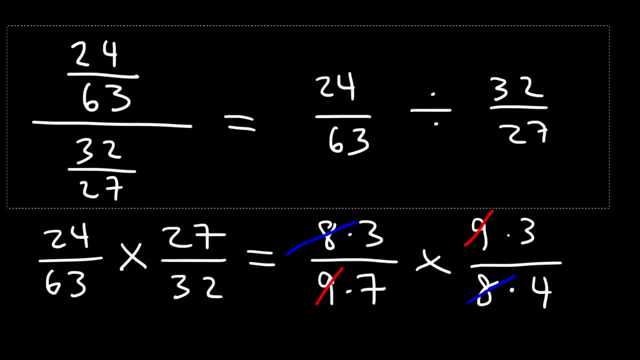 so let's write out what we have left over. so in this fraction we have a 3 and a 7, and in the second fraction we're left with a 3 and a 4. 3 times 3 is 9, 7 times 4 is 28, and so this is the final answer. we can't simplify it any further. 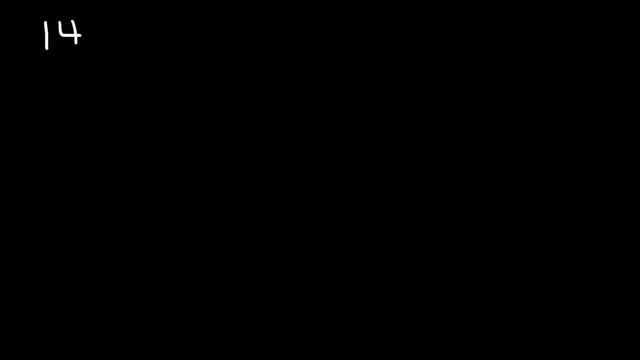 now let's work on another problem, a similar example: 14 over 38, divided by 35 over 57. so go ahead and work on this problem. let's begin by rewriting it just like we did before. so this is 14 over 38, divided by 35 over 57. 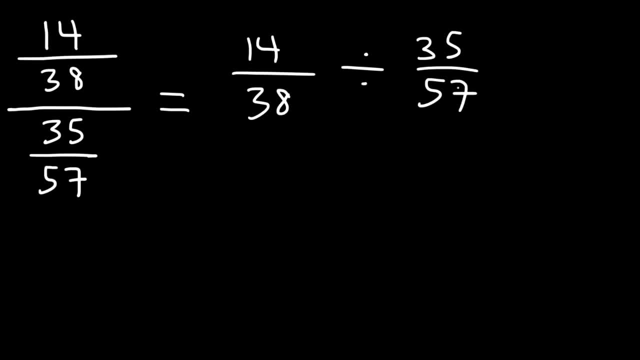 so now let's convert division into multiplication using keep change function. so let's keep the first fraction, the same change division to multiplication, and we're going to flip the second fraction. so now let's simplify before we multiply. so looking at 14 and 35, both numbers are divisible by 7. so I'm going. 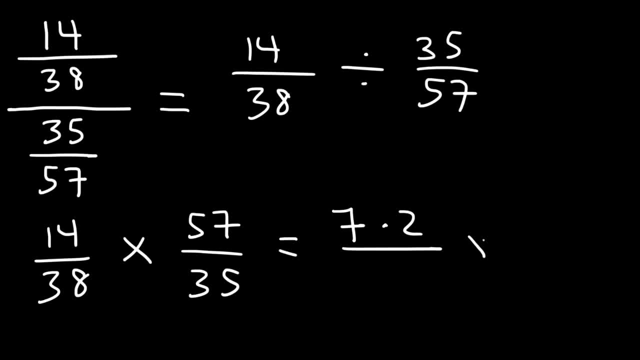 to write 14 as 7 times 2 and 35 as 7 times 5. now, what can you tell me about 38 and 57? now, what can you tell me about 38 and 57? so I'm going to write 14 as 7 times 2 and 35 as 7 times 5. now, what can you tell me about 38 and 57? 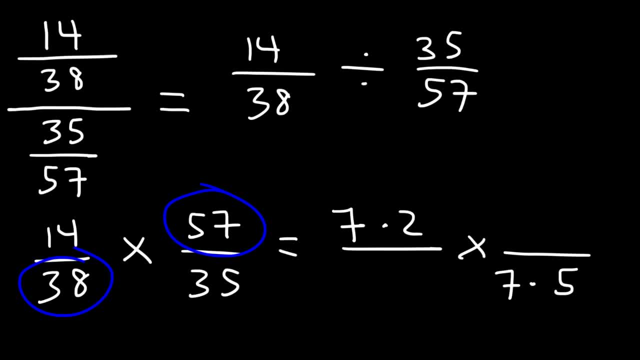 what do you know about these two numbers? looking at them, they're both divisible by 19: 38 is 19 x 2, 37 is 19 x 3, and so we can cancel on 19, we can cancel a 7 and we can cancel a 2, so therefore, 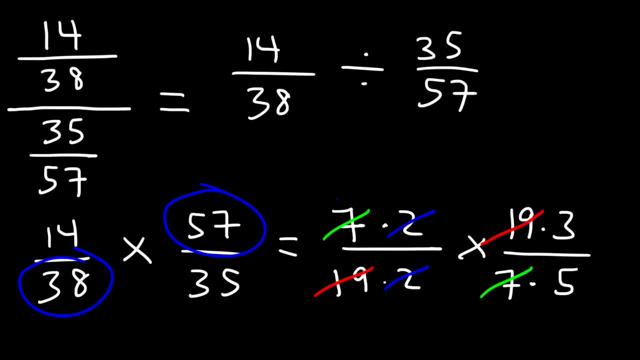 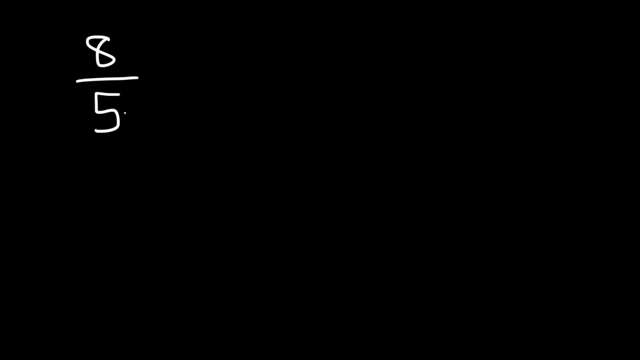 so, therefore, We're left with this as our final answer, which is 3 over 5.. So that's it for this problem. Now, let's say if we have an improper fraction and we wish to divide it by a whole number, like 9.. 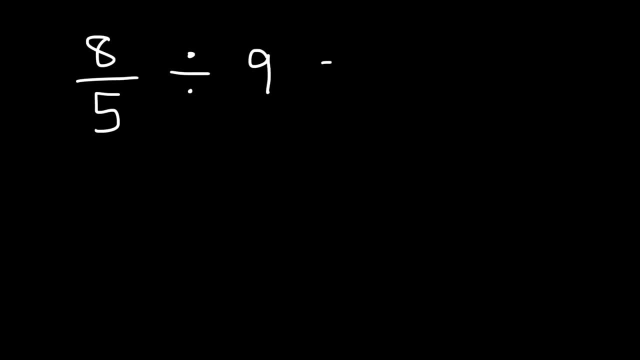 How can we divide a fraction by a whole number? Well, the first thing we need to do is rewrite the whole number as a fraction. 9 is the same as 9 over 1.. And then we can do what we've been doing before: keep, change flip. 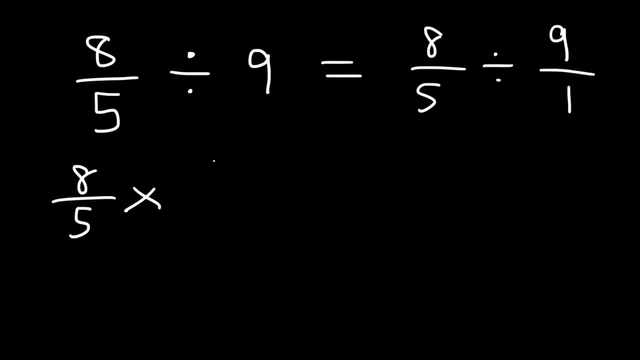 So let's keep the first fraction the same and then change division to multiplication. We're going to multiply by the reciprocal of the second fraction, So now all we need to do is multiply across. 8 times 1 is 8.. And 5 times 9 is 45.. 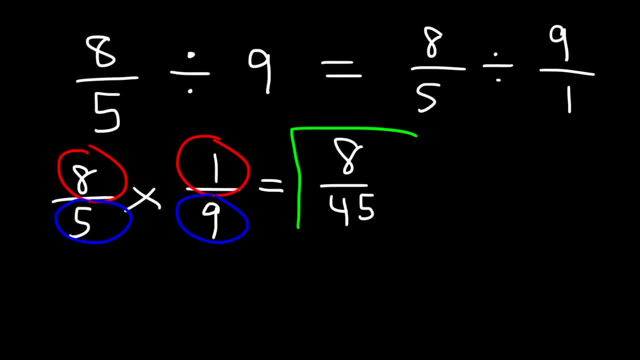 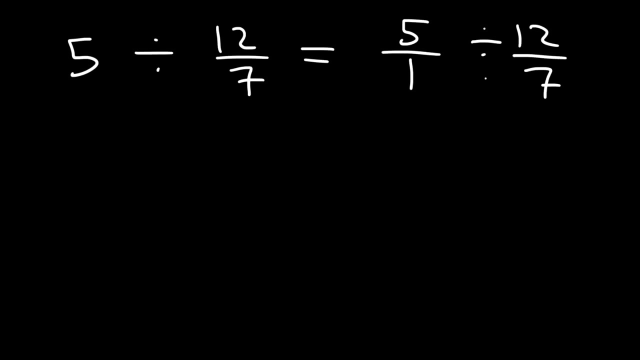 And so this is our answer: 8 over 45, and we can't simplify this fraction. So now, what if we have a whole number divided by a fraction? What should we do? Well, we need to do the same thing: Rewrite the whole number as a fraction. 5 is the same as 5 over 1.. 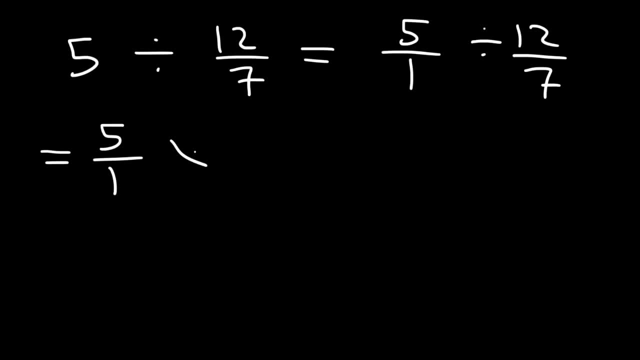 Let's keep the first fraction the same, and then let's change division to multiplication, And then we're going to flip the second fraction. Now we have no choice but to multiply across. 5 times 7 is 35.. And 1 times 12 is 12.. 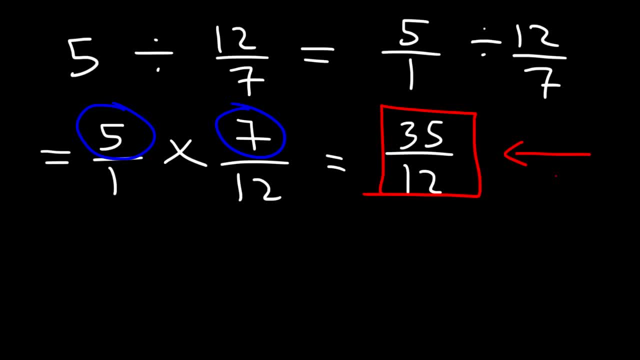 So this is our answer: 35 over 12.. Now, sometimes you may need to convert an improper fraction into a mixed number, And so that's going to be the next video in this series. I'm going to put a link to that video in the description below.